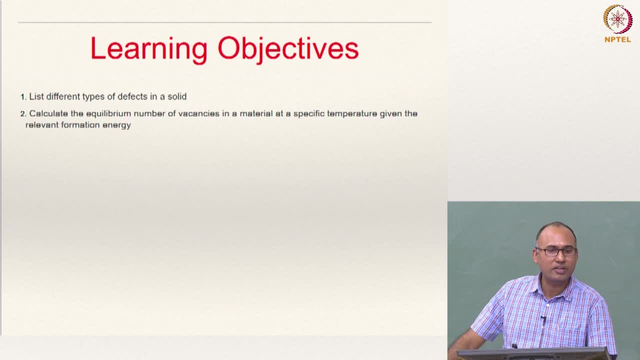 a material at a specific temperature, given the relevant vacancy: formation, energy- Okay, Add different types of solid solutions and give at least 5 examples for each of these types of solid solutions. Okay, And write the conditions for formation of the solid solutions that were listed in point. 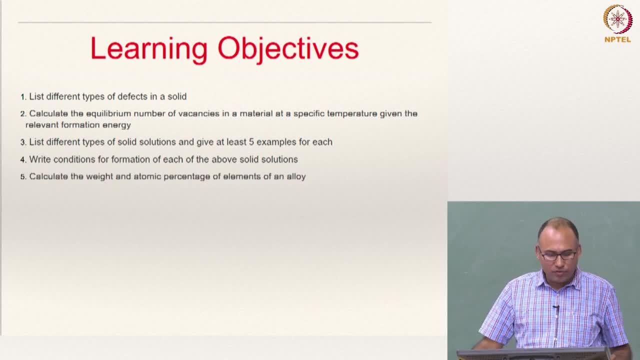 3. And you should be able to calculate the weight and atomic percentages of elements in an alloy and you should be able to convert from atom percentage to weight percentage, the composition. And you should be able to draw the schematics of an edge, screw and mix, dislocations and 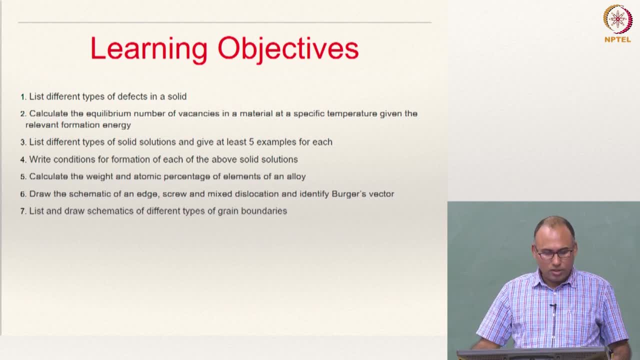 identify something called Burgers vector List and draw schematics of different types of grain boundaries. Explain the role of grain boundaries on dislocation motion. Explain the strength of the nanocrystalline materials compared to their post grain counterparts. List different types of strengthening mechanisms. 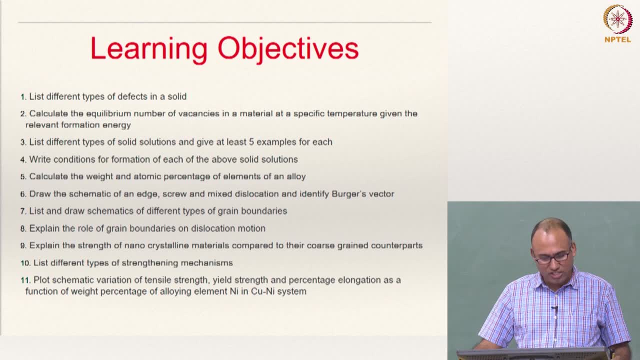 Plot: schematic variation of tensile strength, yield strength and percentage elongation as a function of weight. percentage of alloying elements in nickel in copper nickel system. Okay, Thank you. So these are the three things. So I will get back to you in the next class to learn what I just mentioned. 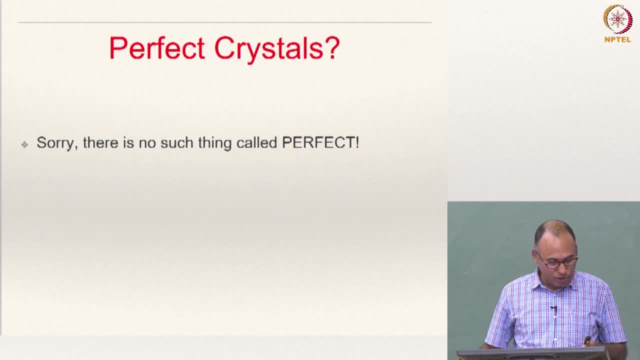 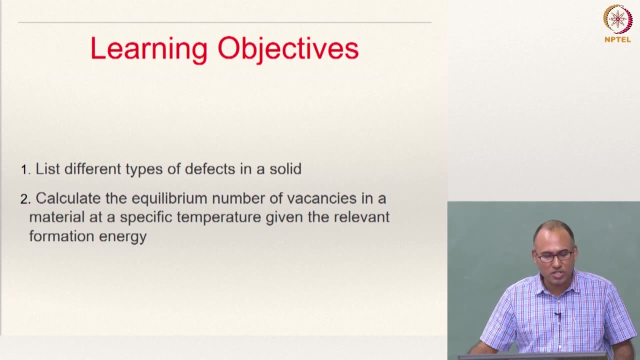 So we have derived the expression for critical, resolved shear stress. So there are how many several learning objectives? So this is a very important topic. This is this actually helps us understand the deformation mechanisms that we have discussed. We will talk about in future in the last class. 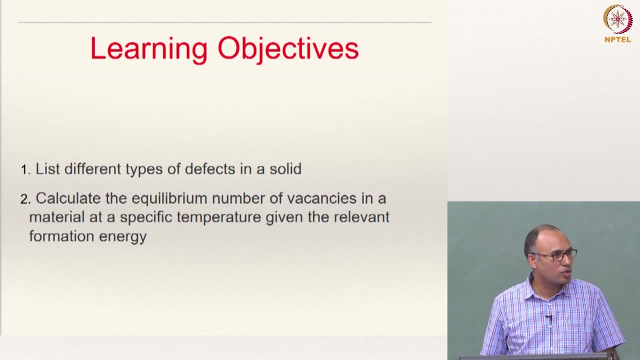 Right, So this chapter, this topic module, lays the foundations for the deformation mechanisms. right? So this topic module lays the foundations for the deformation mechanisms that we have discussed in this lecture. right, Thank you, Bye, Bye, Bye, Bye. 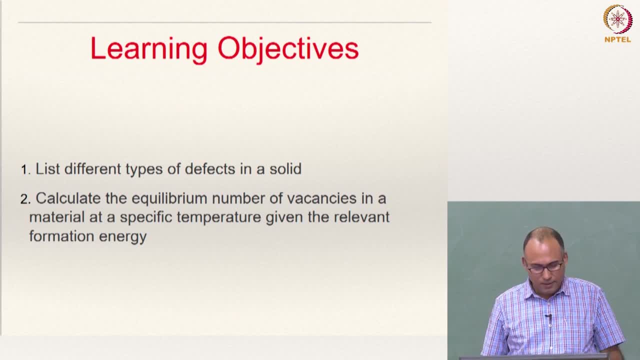 Bye, Bye, Bye for understanding the deformation mechanisms, okay. So in this class we will try to achieve these two learning objectives. The list different types of defects in a solid and we should be able to calculate the equilibrium concentration of vacancies in a material at a given temperature, at a specific temperature. 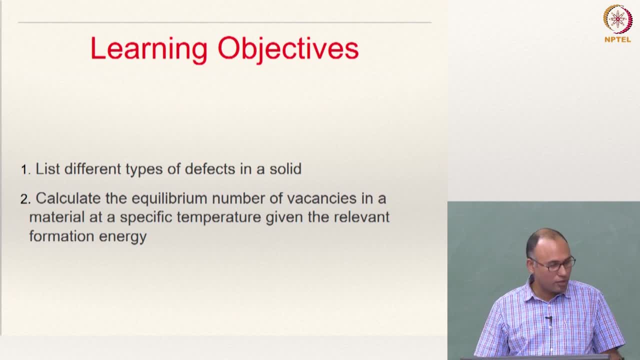 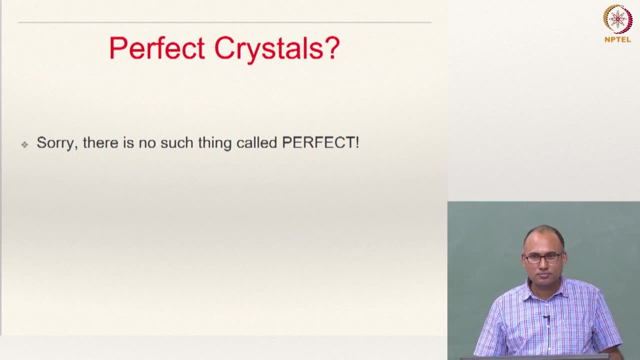 by knowing the vacancy, formation, energy of that particular material. okay, So perfect crystals. are you familiar with any perfect crystal? Unfortunately, there is no such thing called perfect. perfect crystals do not exist. So in some sense, philosophically if you want to say, materials and human society are alike. 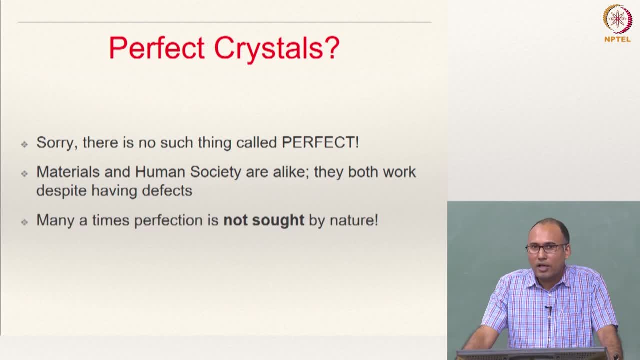 They both work despite having defects, and several times it is actually desirable not to have perfection. We may think that perfection is always good, But sometimes it is sought after. imperfection is sought after, we will see in, particularly also in mechanical engineering applications. the defects are one of are very important. 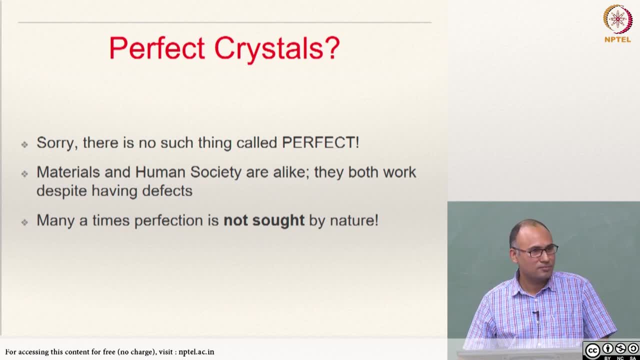 for us to actually make several things right. So if you want to make a sheet metal, how do you make a sheet metal? you must have studied in your manufacturing technology or manufacturing processes: Okay, How do you make a sheet metal? So we actually have a billet and then run the billet, iron billet or whatever, aluminum. 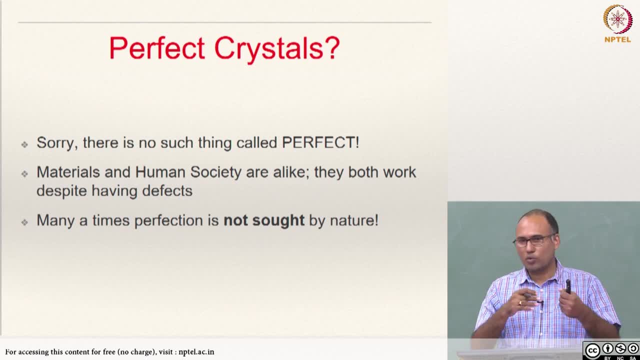 sheet, metal whatever, and then run between two rollers and then it becomes a sheet. A solid block can be made into a sheet. The reason why you are able to make that into a sheet is because the sheet is made of solid. it is made of solid. you are not going to have a solid block made of solid sheet. you 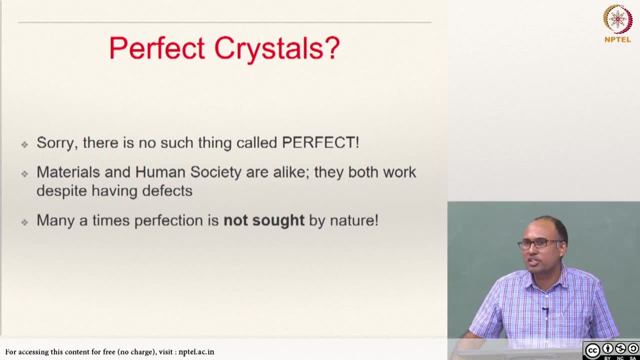 are not going to have a solid block made of solid sheet because you can impart plastic deformation in the material. Imagine if the material is brittle. That means it will simply break. You will not be able to impart such huge amount of plastic deformation. 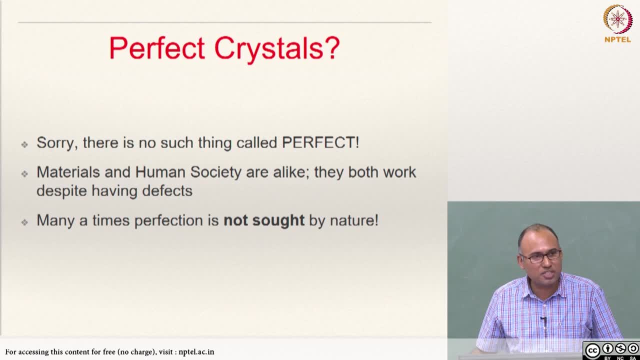 And if not for defects, you will not have plastic deformation, You will not be able to impart plastic deformation Right. Plastic deformation is actually the motion of one kind of a particular kind of defects in material called dislocations, Right. So in that sense, 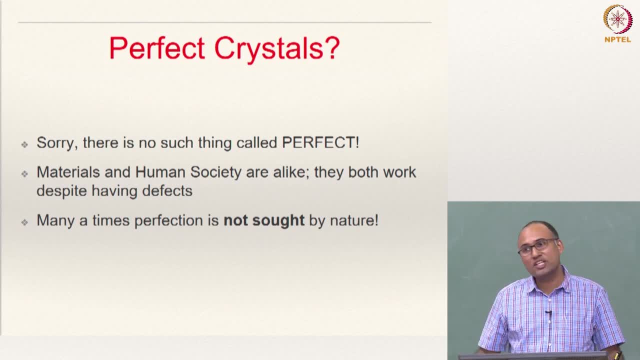 several engineering components can actually be made because of the presence of defects. So many times perfection is not sought after And they actually will lead to many good things. The best example is semiconductors. Right Semiconductors work because of doping. 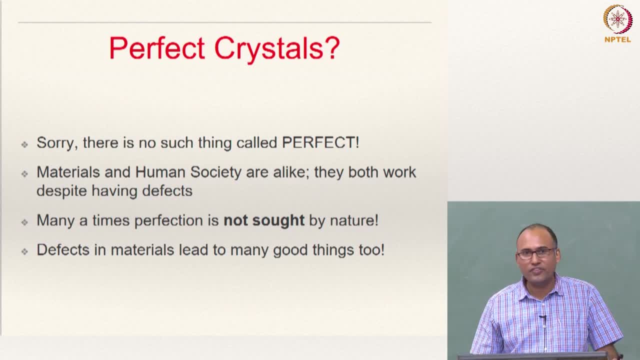 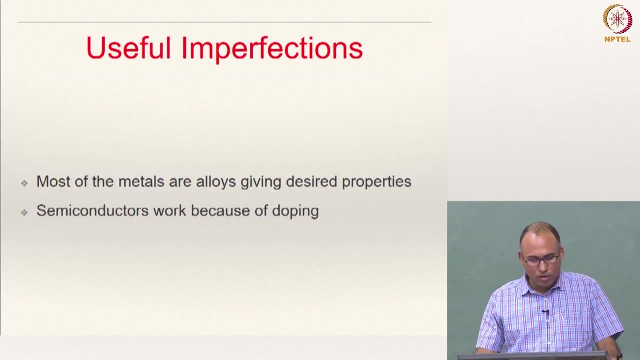 because of adding impurity elements. So you're adding some defect to the material intentionally to get something very nice out of it, Right? So useful imperfections? Mostly, most of the metals that we are familiar with are alloys. That means you don't have pure material. 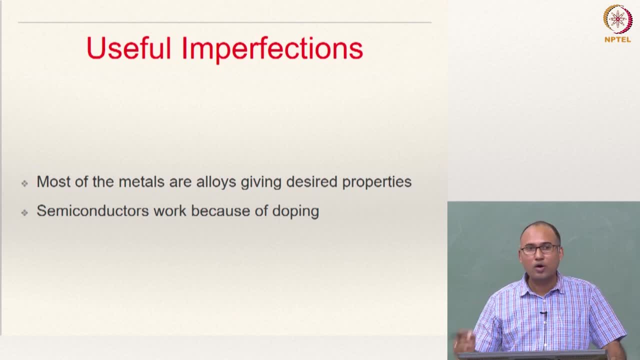 It's impure, It is not pure. That means it is not only one element. For instance, if you take steel, steel is an alloy. of steel is an alloy of iron and carbon primarily, And there are there are going to be other elements too. 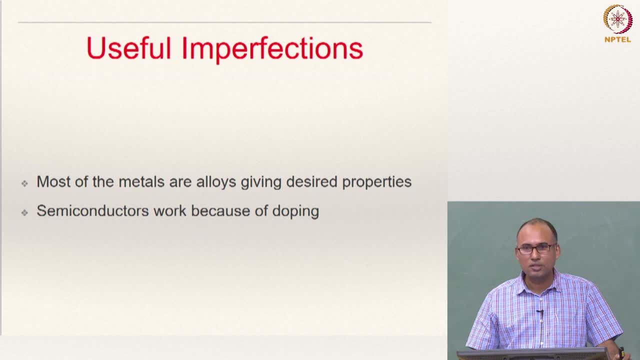 So, but it's not purely iron, Right? If it is purely iron, you probably won't get, you won't be, probably won't be able to get the properties that you are actually enjoying with steel. So alloying is something that you are actually making. 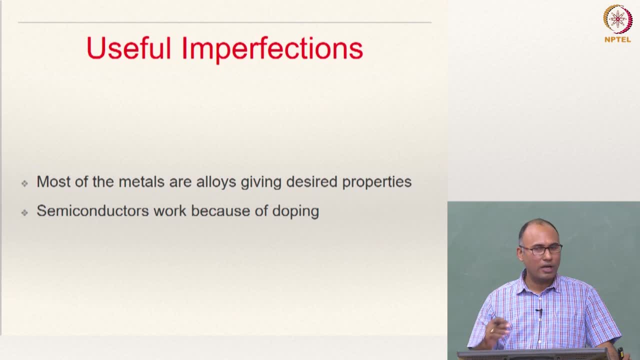 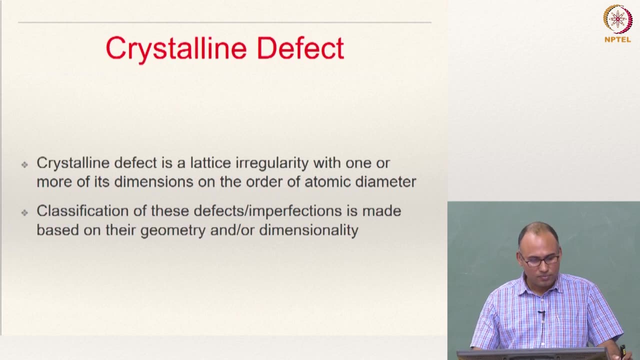 a pure material, like iron, as an impure material by alloy, adding other elements, But getting good things out of it Right. Similarly, semiconductors. So now we need to define. what do we mean by a crystalline defect? 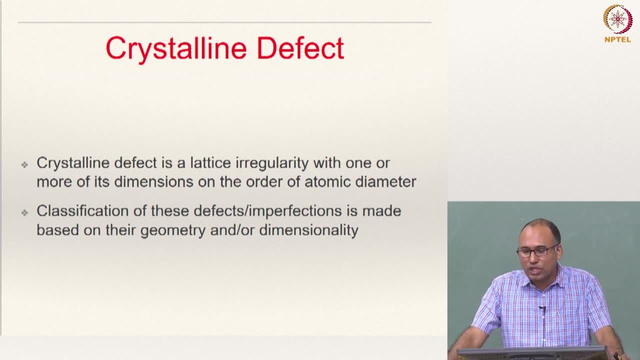 So the crystalline, a crystalline defect, is a lattice irregularity with one or more of its dimensions on the order of atomic diameter Right, It's a lattice irregularity. So how do you classify these defects? So that means there is some irregularity in the lattice. 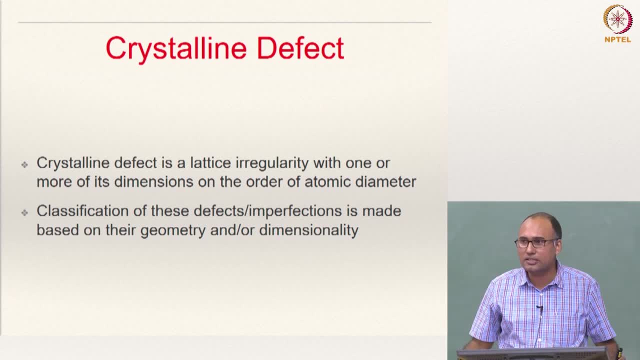 So that means there is some irregularity in the lattice. So that means there is some irregularity in the lattice, in the lattice structure that we have discussed in the previous chapter or previous module, right? So what are the? how do you classify these defects? They can actually be classified based. 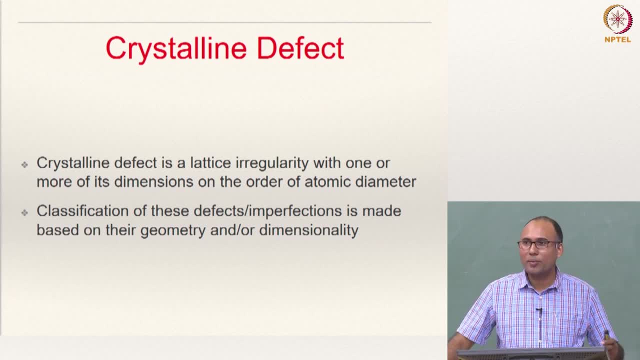 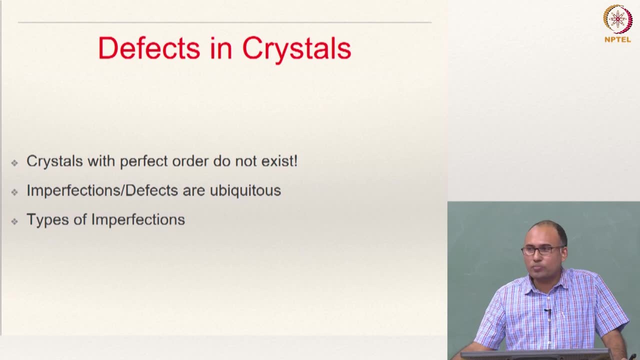 on the geometry of the, or geometry or the dimensionality of the defect that we are talking about. So, as we are discussing, crystals with perfect order do not exist. Even if you want to, they do not exist. We will see in a moment why they do not exist And imperfections or defects. 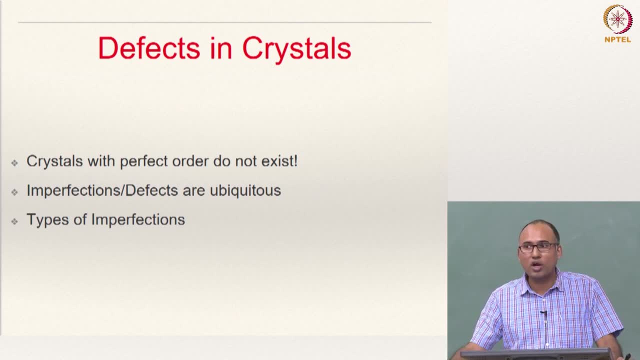 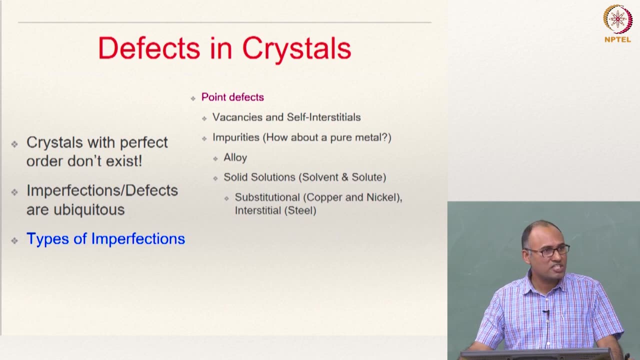 are there everywhere. And what are these different types of imperfections or crystalline defects. The first kind of defects are called point defects, So zeroth order, dimensionality, right. So what are these point defects? For instance, if you have a crystalline lattice, 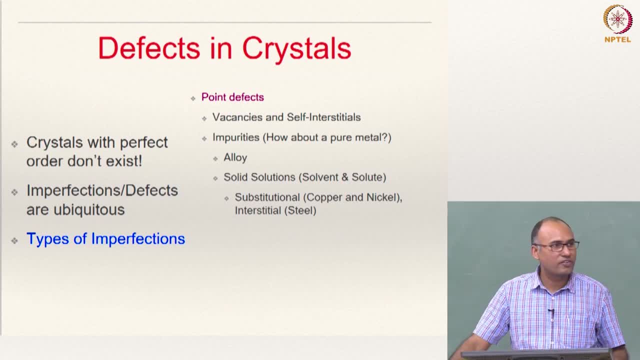 if you have a vacancy or self-interstitial. that is one kind of a defect. Vacancy means if you need to have an atom there but you do not have one. That means a lattice site which should have been occupied by an atom or a molecule is not occupied by that motif. So 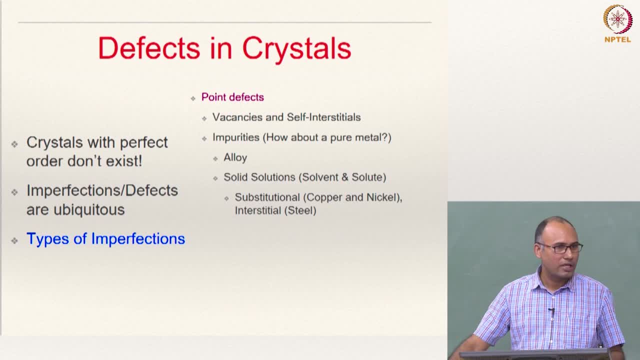 basically you have a lattice site but you do not have a motif. Every other place you have motif, but at that one particular place you do not have the motif. Then it is a vacancy And a motif has specific position to sit in right the lattice sites. But if the motif goes, 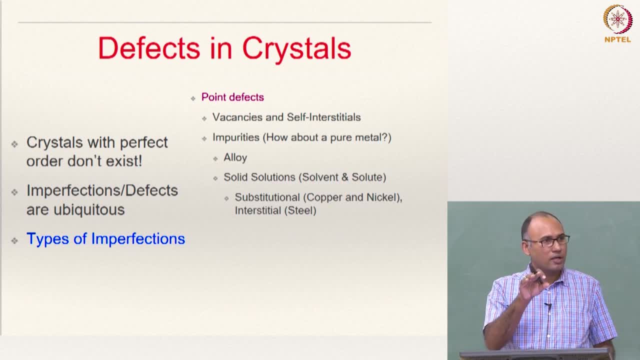 and sits in some other position which is not its lattice site, that which is where it is not supposed to be sitting. that is also another kind of defect. So that is going and sitting in a place where it should not be right. So all of you have here lattice sites. 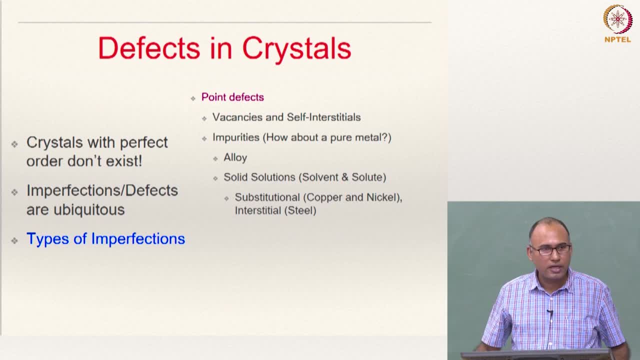 and you have here all different motifs. right for this classroom. And you are not expected to sit between the benches. If somebody comes and sits in between the benches, then he or she becomes the point defect for this nicely ordered class, right. 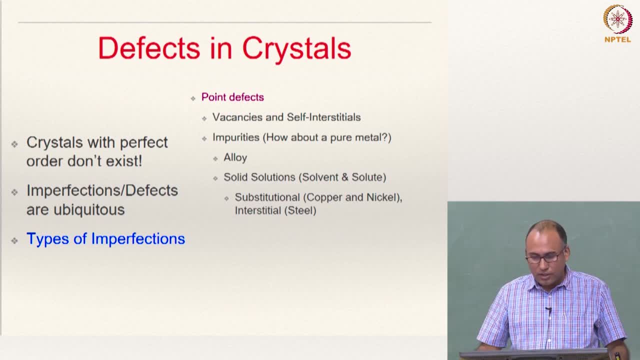 So that is what you mean by point defects, right? You can also have impurities, which means normally you have a crystalline lattice such as iron, And then there is another impurity comes and sits in the crystal lattice And that is what makes it an alloy And you have you have this kind. 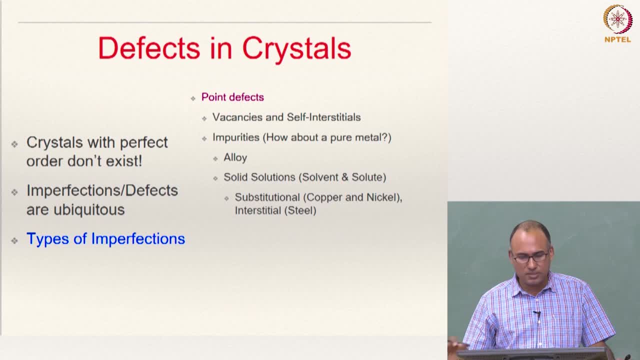 of material called solid solutions, which we will discuss towards the end of this course. what different kinds of solid solutions? And then the next level of defects are called line defects. So, according to dimensionality, the first one is zeroth order And the second one is first order. 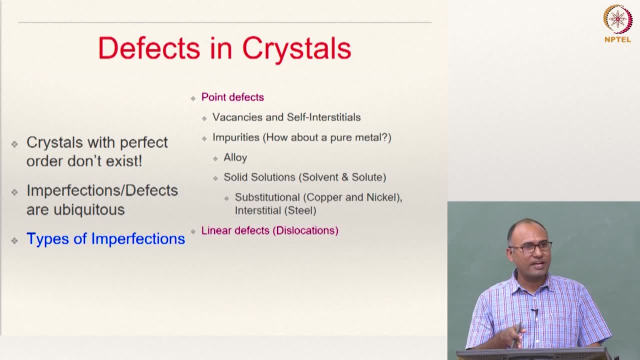 second order and third order. So like mean? that means point defects, line defects, next will be area or surface defects and then will be volume, 0 dimensional, 1 dimensional, 2 dimensional and 3 dimensional. So the line defects or linear defects are also called dislocations. 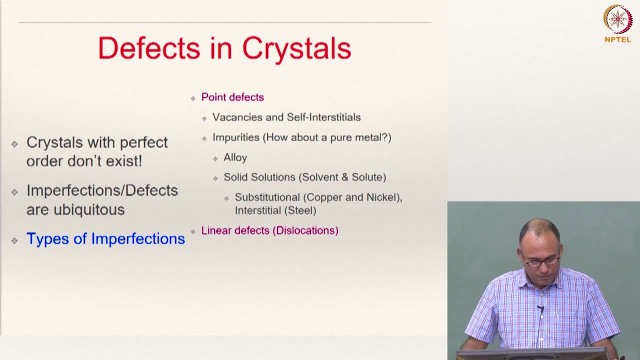 That is what we will look at in detail in this course. And then you have interfacial defects or 2 dimensional defects or surface defects. right, So you have, they have 2 dimensional description. So they are external surfaces: grain boundaries in a polycrystalline material. 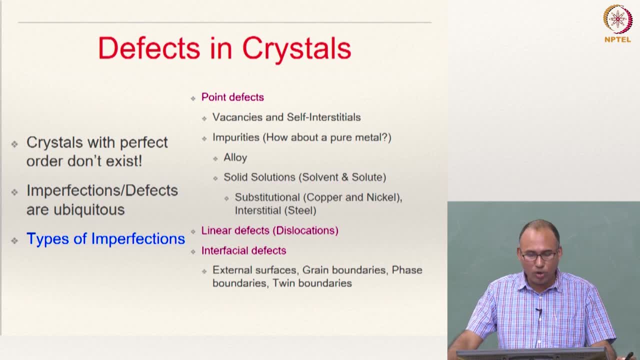 So grain boundaries are sort of defects And face boundaries fin boundaries. we will see what they are. And then you have bulk or volume defects, which means you have a crystalline material from the bottom up And if you make your big actual structure normally you would expect your atoms to be 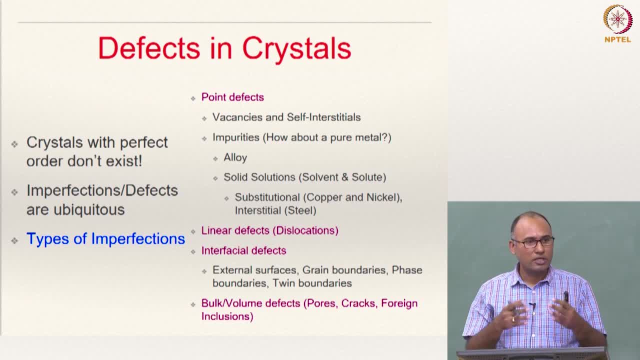 filling the entire space And sometimes in your material you may find some voids pores right. it is a 3 dimensional defect where there is nothing. The material is not present for some reason or some. due to some reason that during the 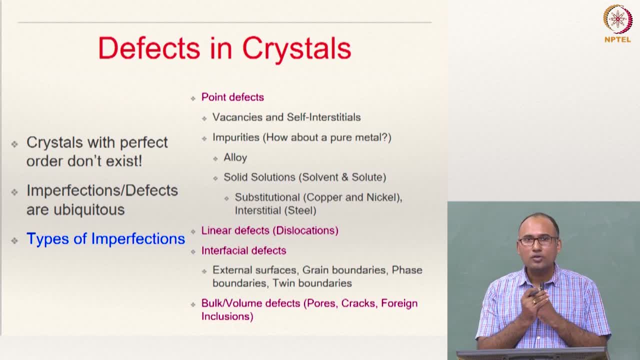 processing of the material, this pore comes in right. So this is a 3 dimensional defect. Similarly, cracks and foreign inclusions which are not supposed to be there in the material. So these are all the different kinds of defects that you have in a material: point defects. 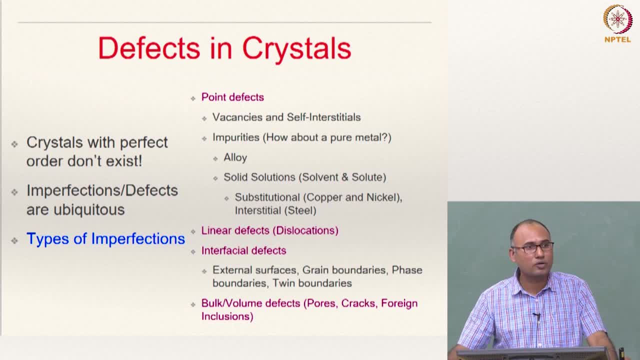 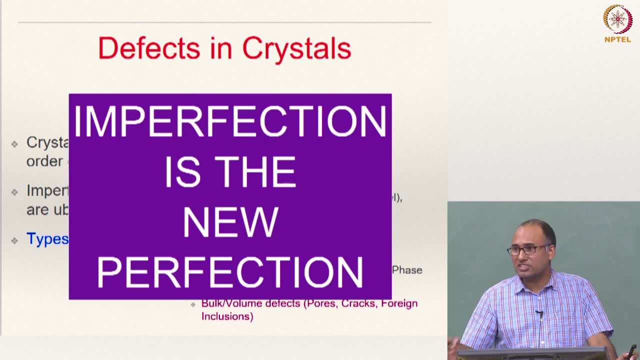 line defects, interfacial or 2 dimensional surface defects. So these are all the different kinds of defects that you have in a material: Two dimensional surface defects and volume defects. okay, So, as we have discussed, imperfection is something that is not necessarily a bad thing, okay.